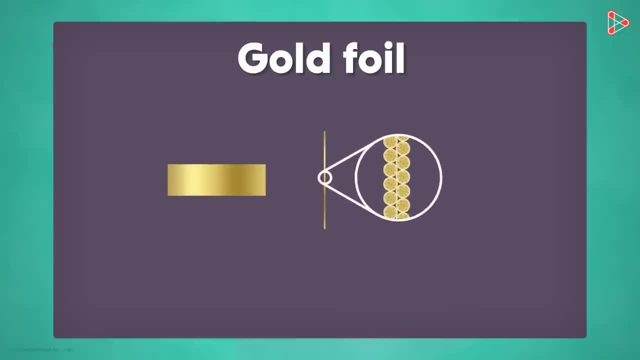 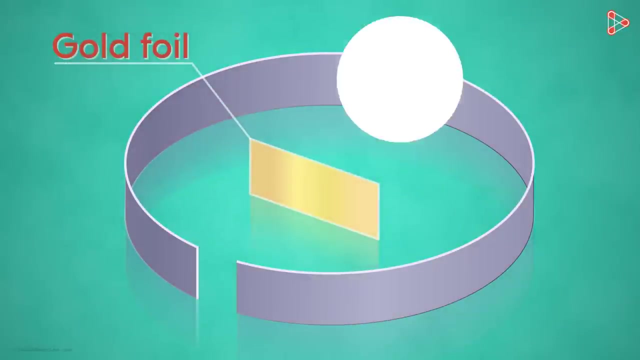 Why did he choose a gold foil? Well, a really thin gold foil was estimated to contain approximately 1000 atoms. Lesser the atoms, more convenient the experiment would be. Lastly, are we able to locate this circular band with a gap here? 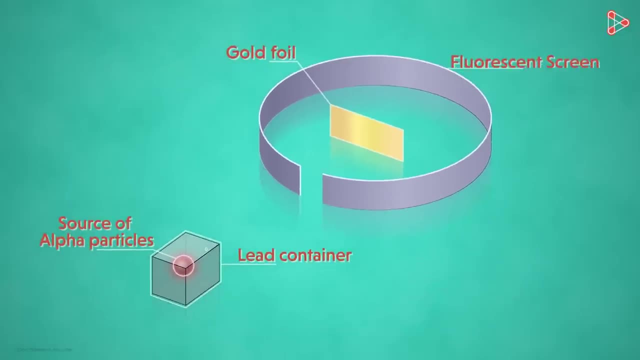 What could this be? Well, this is a screen, A fluorescent screen that would help us detect the radiation. Ok, That means the screen will glow or emit fluorescent light whenever alpha particles will hit it. So this is how the track of alpha particles can be traced. 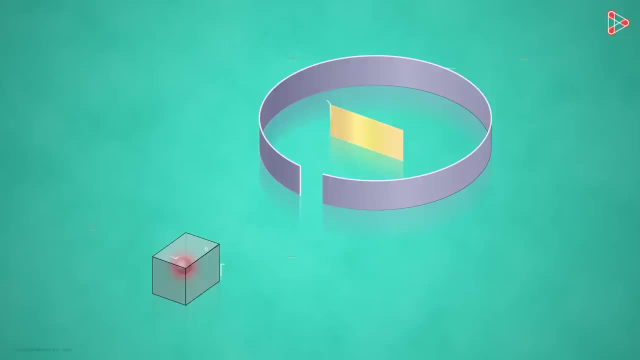 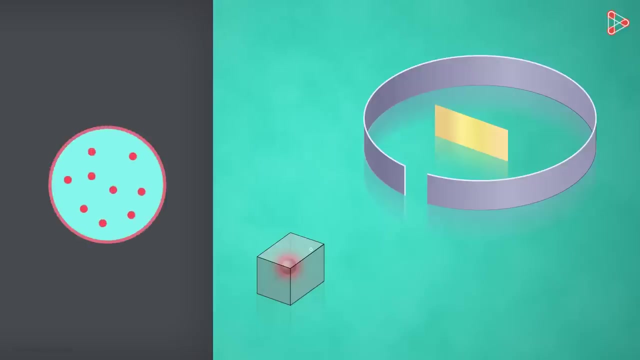 Now we are all set to understand how the experiment worked. The alpha particles were emitted from the element present in this box. These directly hit the gold foil. Now what should happen ideally? As we know, the Thomson's model suggested that an atom is a sphere of positive charge. 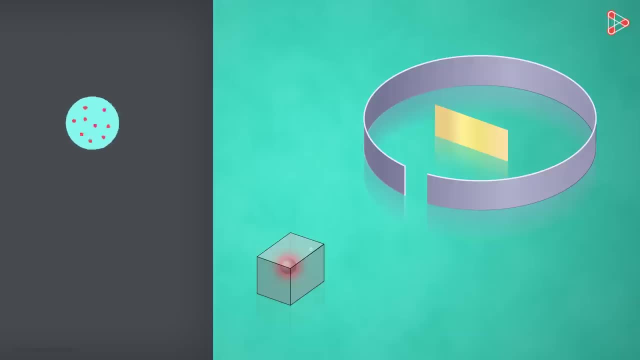 with negative electrons in it. That means it is expected that the alpha particles will pass right through the atoms and hit the detector straight. And why so? Because the mass of alpha particles is heavier than the mass of positive charges. That means they should directly hit the atom and move ahead through it. 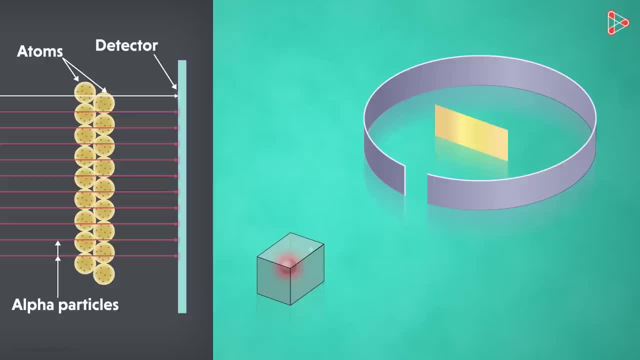 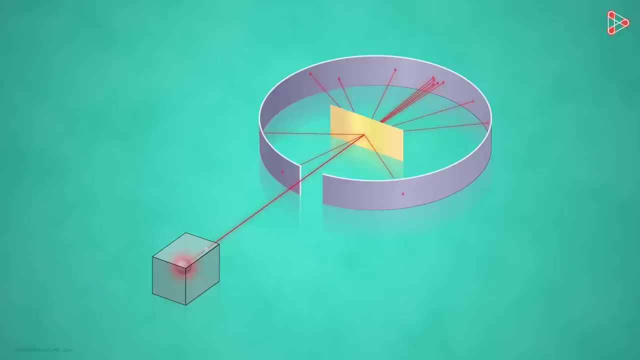 Only a very small deviation would probably be acceptable in this case. But is this what he observed? Not really. He was astonished to get unexpected results. What results did he get? He found that most of the fast-moving alpha particles passed straight through the foil. 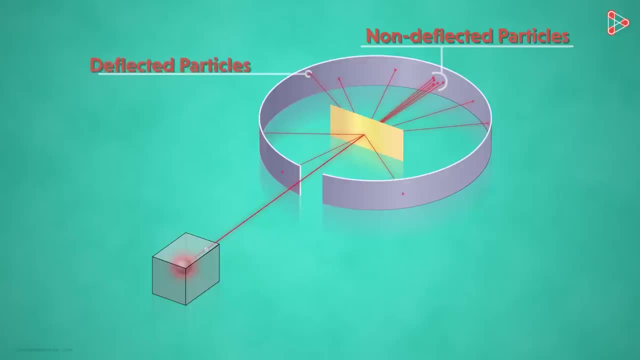 and hit the detector. However, some particles got deflected by small angles And lastly, to his astonishment, few alpha particles also rebounded. Now, how can this be possible? These three observations made Rutherford think that the plum pudding model is not true. 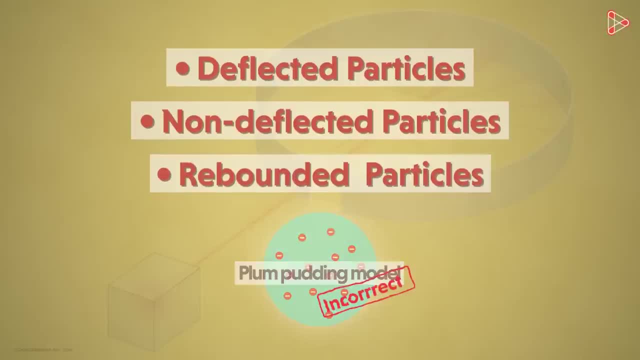 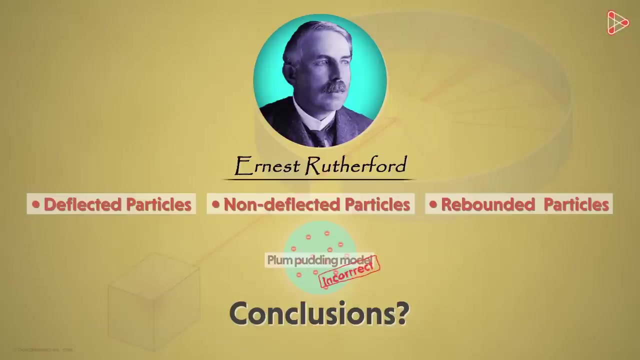 Now, what is the answer to this question? Let us find out. Let us find out. The answer is not really correct. Based on the conclusions he had, he put forward the new hypothesis explaining the structure of atoms. What were his conclusions? Let us have a look at the conclusions by Rutherford, followed by the new atomic model put forth. by him in the next video.